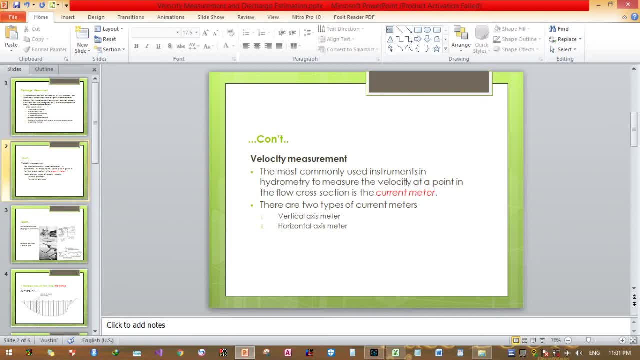 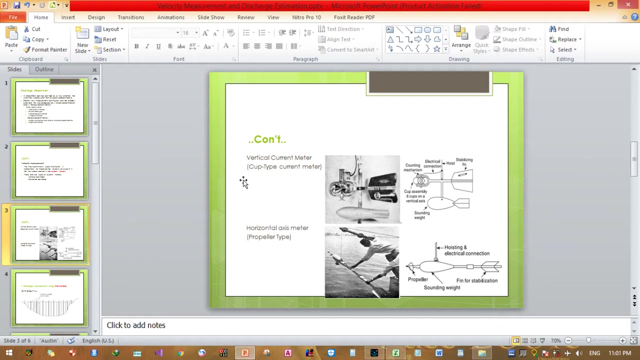 These are instruments used to measure velocity at a point in the flow. There are actually two types of current meters. The first one is vertical axis meter And the second one is horizontal axis meter. So in image we can view this type For vertical current meter. there is an example of cup type current meter here. 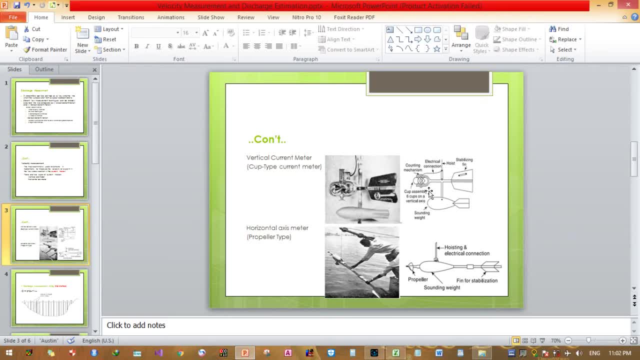 This is each section of this cup type current meter, illustrated here in detail. There is a cup assembly, six cups on a vertical axis. This is sounding weight, This is electrical connection, This connection unit, This is host, Stabilizing fin. 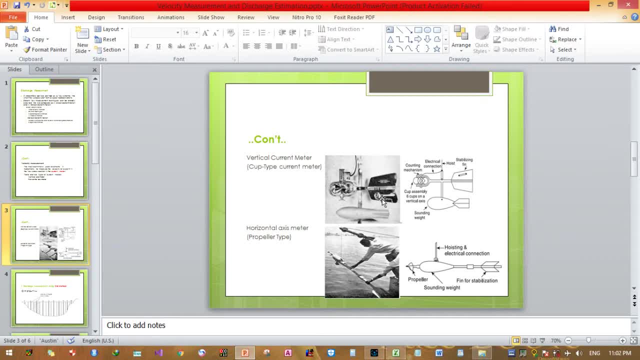 This is fin, Which stabilizes this sounding weight. There is accounting mechanism here. Accounting mechanism is available here, Whereas the second one is horizontal axis current meter. This is a propeller type of horizontal axis meter. This is an illustration. This is a hosting and electrical connection. 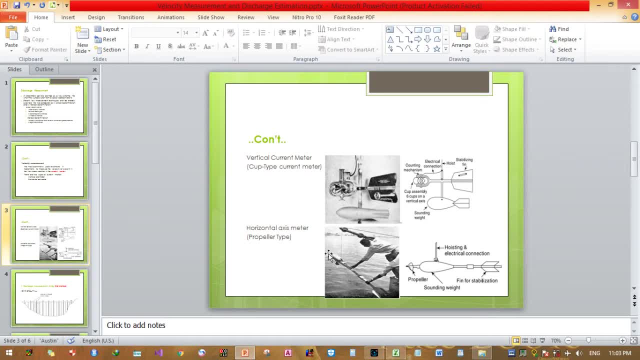 This is surrounding weight, sounding weight. The front one is propeller Here. as you can see, this is propeller. It rotates. This is fin for stabilization. Likewise for vertical current meters of cup type current meter. This is a fin here. 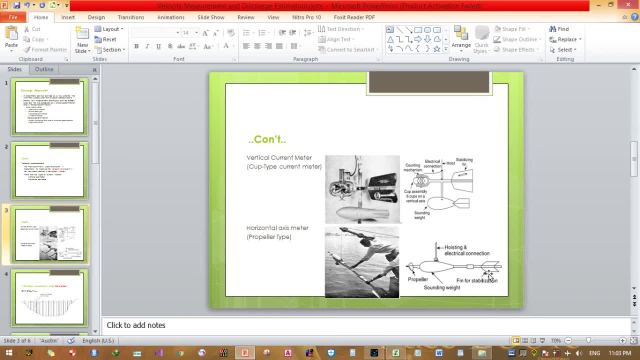 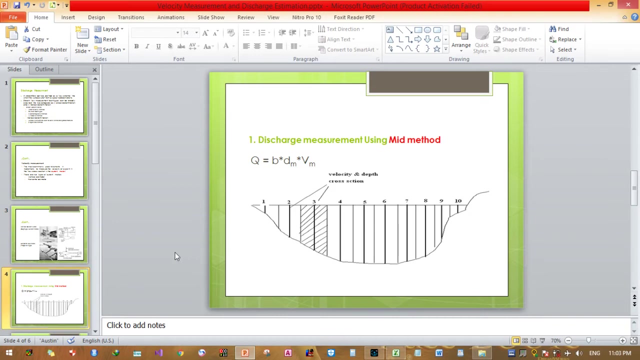 It's also available here, A fin type. The only difference here is this cup assembly: Six cups on a vertical axis are assembled in such a way. This is horizontal, as you can see. Propeller in the front is horizontal as well. Now let's look at those discharge measuring using mean method and mean method. 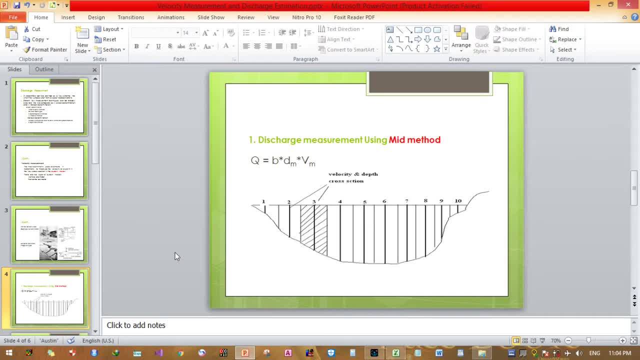 Therefore, the first one is discharge measurement using mean method. Using the equation, Q is equals to, or stream flow, or discharge is equals to width of individual slice times depth of average. The second one is average velocity. Therefore, using mean method, If this one, two, three, four, five, six, seven, eight, nine and ten. 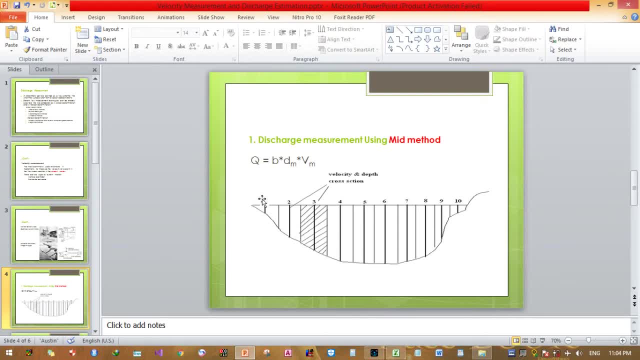 These are depth gauging station as well as velocity gauging station. Then by just taking average of this- two and three in the middle and three and four in the middle- Then we can determine the flow through this slice. This is slice. 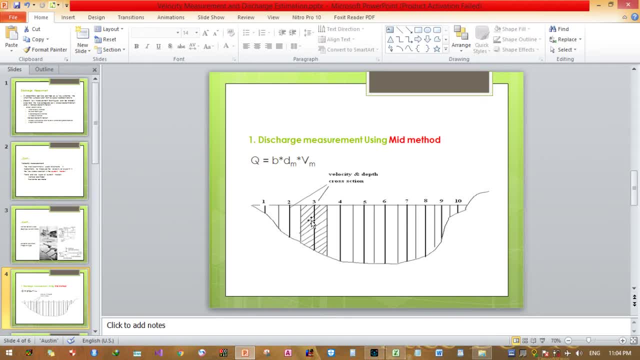 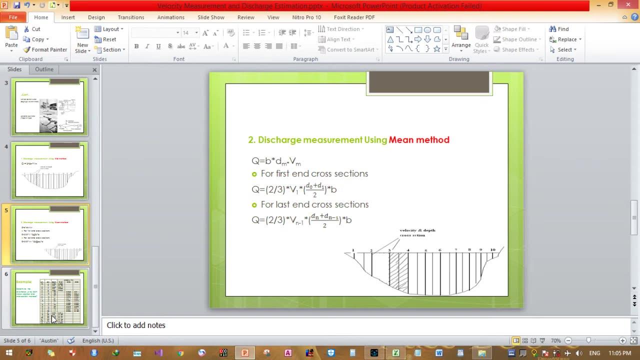 This hatched slice. So this is overall concepts for discharge measurement using mean method. The other one is using mean method. You can determine discharge using in such a way: Q is equals to width times, diameter, mean times, velocity, mean For first in the cross section and for last cross section. 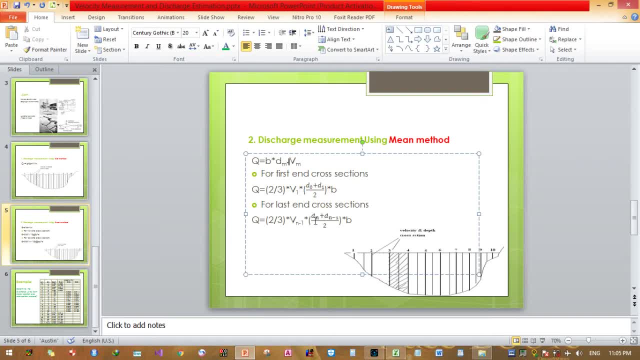 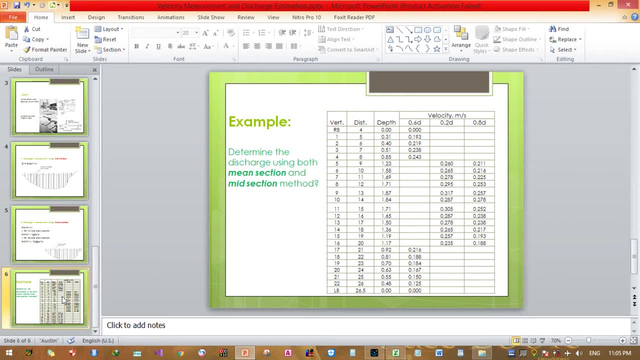 You can determine the discharge using these two equations. So now let's look at- Let's look at this example for identifying those two meters: Determine the discharge using both mean section and mid section meter. This is the given one, So let's copy this one. 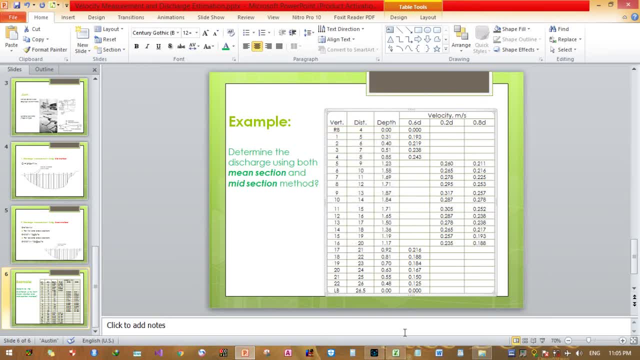 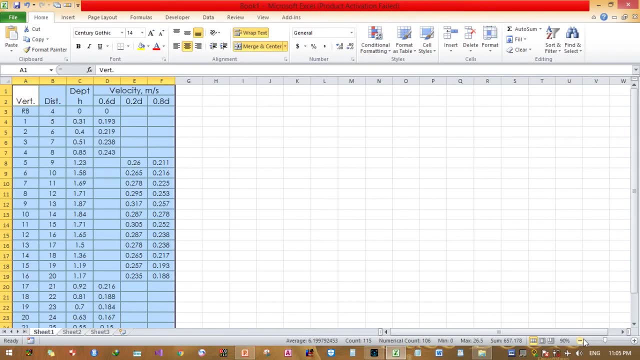 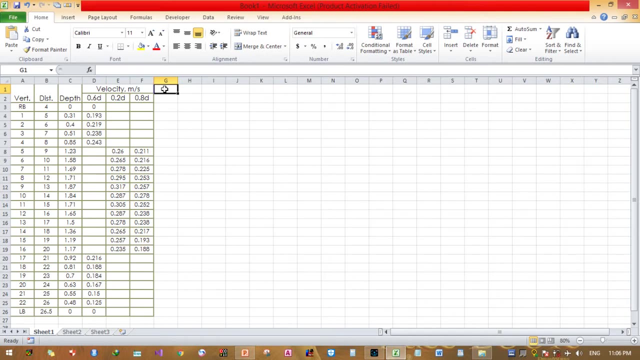 Into axial and direct, determine Discharge. Now we need to find velocity for mid and mean, Velocity of mean section. This is equals to Velocity mid and here velocity mean. Now, as you can see, These are velocities, These are depths. 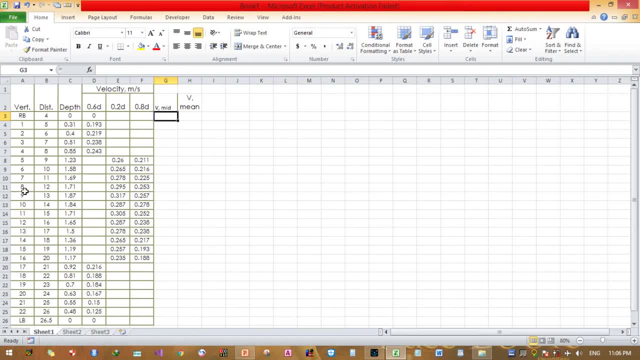 This is distance And this is symbol for right bank and left bank And overall sections here, Point one, point two, At a distance of six. These are symbols, These are real distance From right bank. This is velocity at zero point, six times dips. 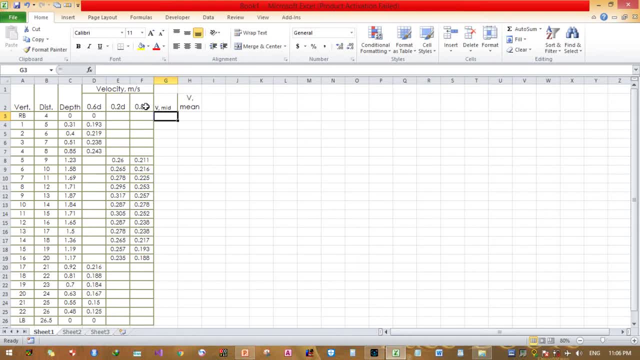 These are zero point two times dips And zero point eight times dips. So these are gauged Value, Measured dips actually. So Measured dips velocity, These are velocity actually. So this is zero point two. six, For example, is: 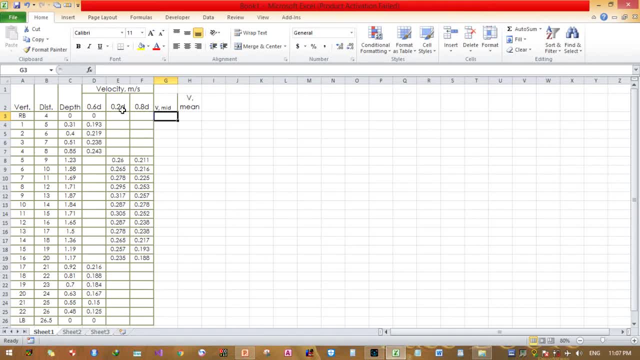 The velocity at a dips of zero point, two times D, Where D is At a dips of zero point, two times this one, This one. This is. This is the velocity. So At this dips, The velocity is this one. This is the total. 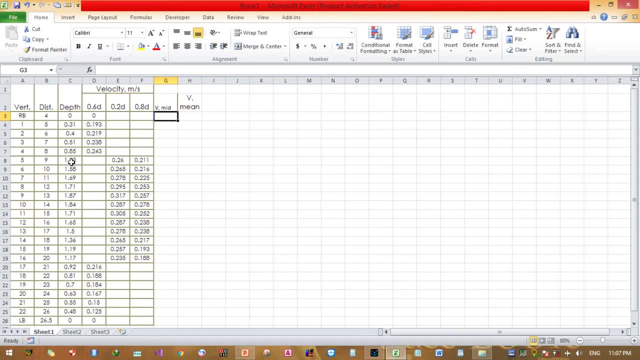 Actually At zero point two times of this dips Velocity. is this one At zero point eight times This dips Velocity. is this one? Therefore, V according to mid Mid Method Velocity is equals to: For this section It's equals. 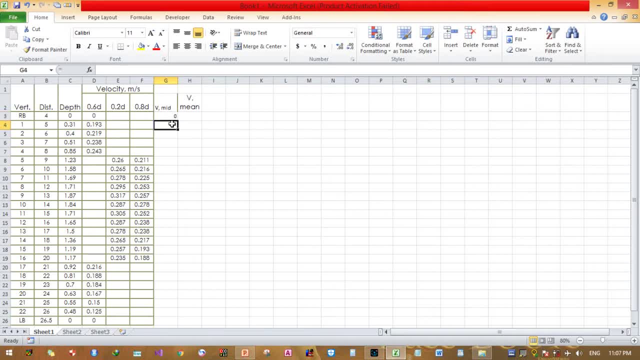 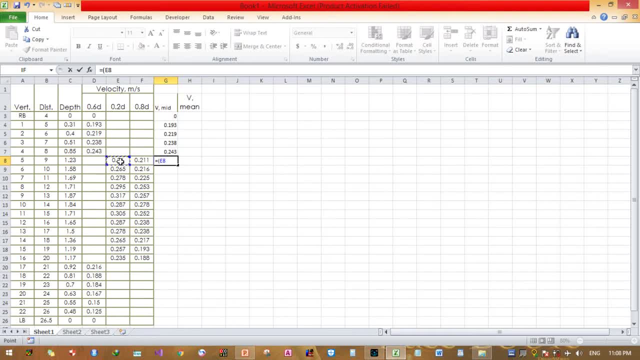 This one, This one, Bracket This one, This one, Pls, This one, Divide by Two, Then press delete window And ah, The same applies to Ah, All Till this One. So In the 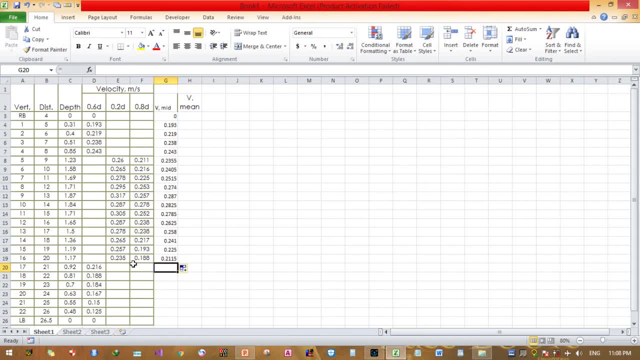 Last one, The velocity. only. Velocity is Zero point six Times this. Therefore We will tuck Tuck Without Averaging. Now We can drag also Here, Here. and this is the velocity at mid section. 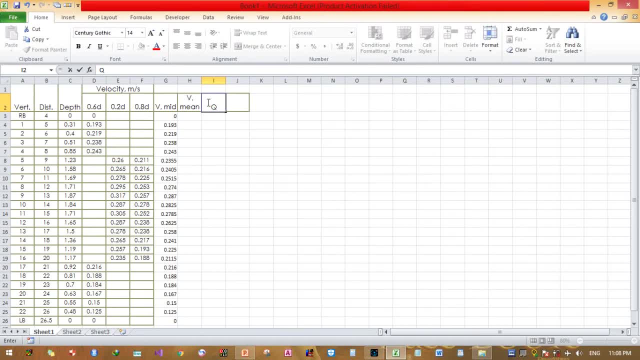 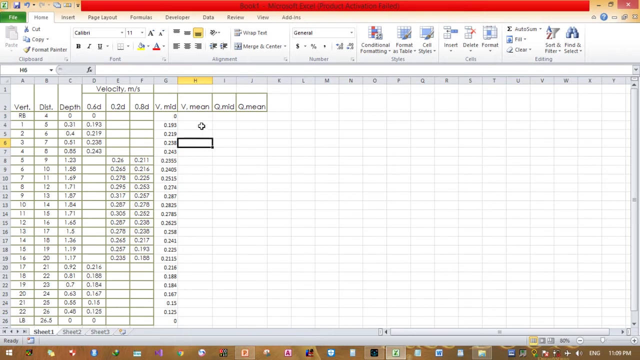 so here discharge using mid section. here discharge for mid section. Yeah, now you here. velocity according to mid update. she said: 0 for this one equals to this one. sorry, bracket this one plus the first one and average divided by two, i think i think. so now drag this one till this one. 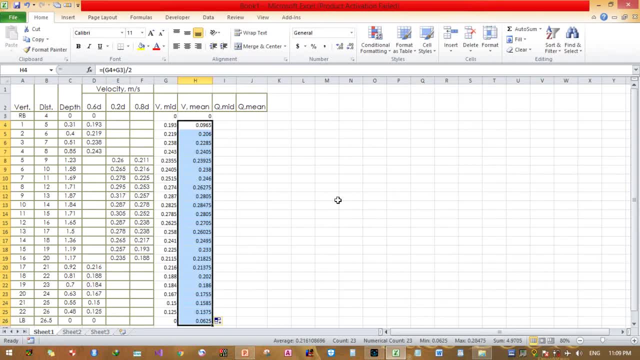 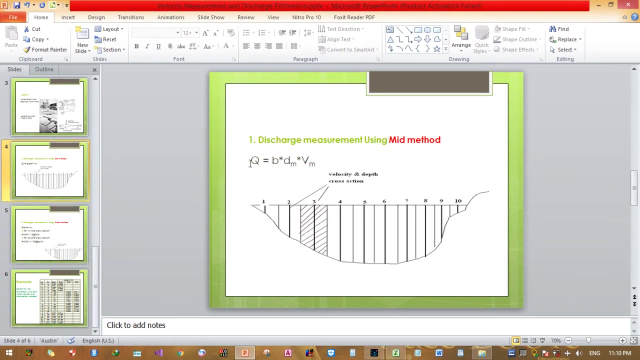 till this one here. this is a velocity using mid main section as well as- uh, it was using a midsection, so then we can. we can compute this midsection for the first one, for this one here, according to cube loose midsection method. this is midsectionated. 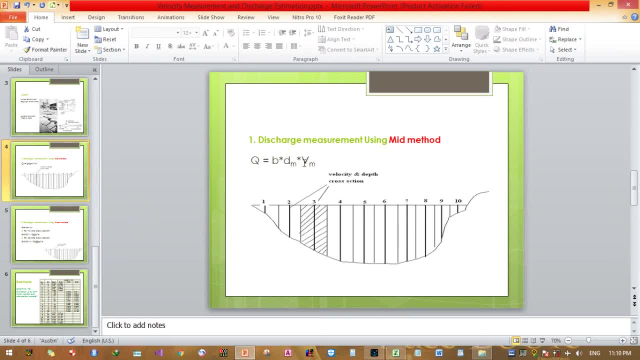 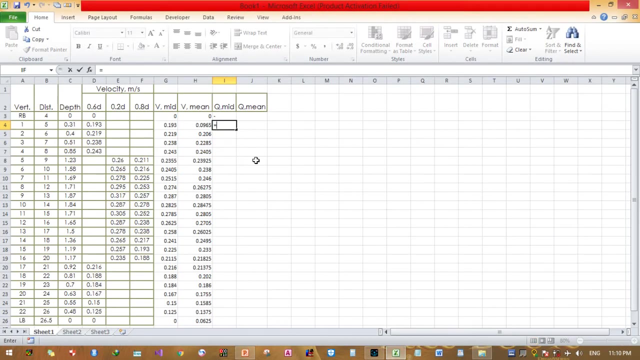 equal to width times, depth times, velocity, average velocity, mean mid. this is mid, not mean mid, velocity mid. therefore, here go here. it's equal to width from 5 to 4, 6 to 5. we can subtract from 5 to 4. this is 1, therefore constant 1 here. 22 minus 21, 1. therefore you can also add 1. 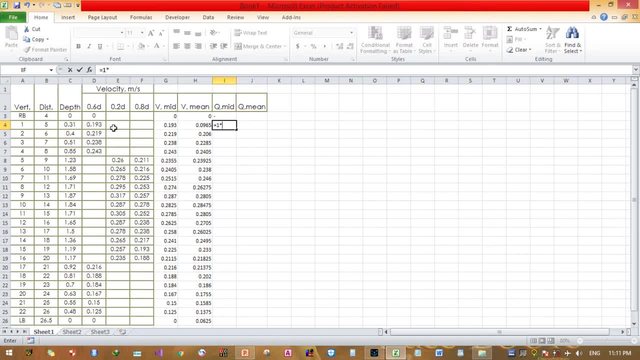 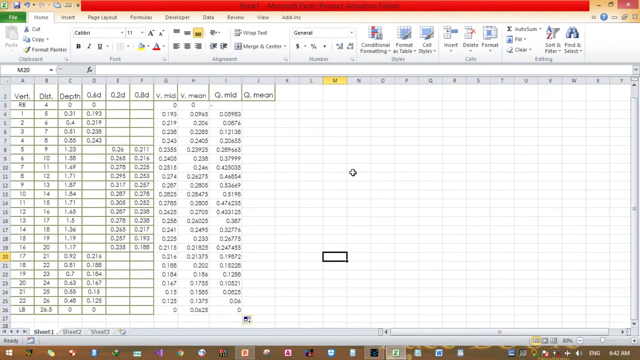 times depth. depth as this one. this one is the depth times velocity mid. therefore, use this one, hit enter now. this is the discharge here. you can also drag this. now you can edit our team. now we will see how we can fill using mean method. so the first one is the vertices and the second one, and this is the second one. 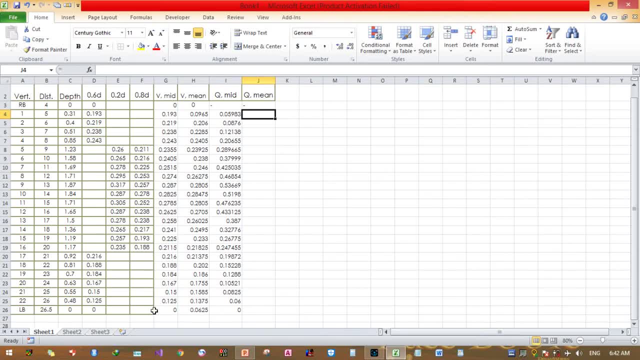 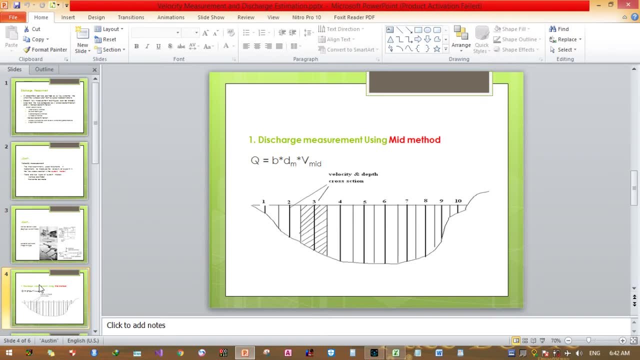 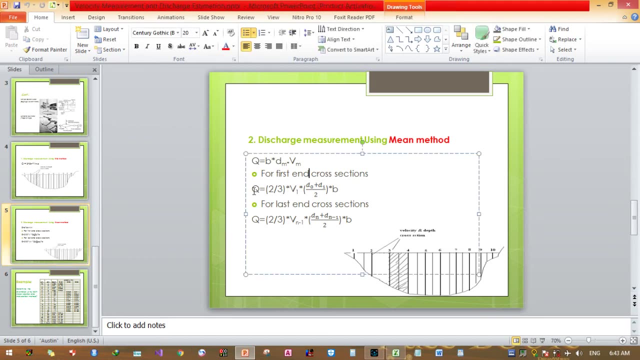 which is the end for the first, and this is the end for the last. so we will see how we can fill using mean method. this is mean method for the first cross section. we can fill the discharge using this equation: two over three, multiply with velocity, one at the depth, one, then there's average. 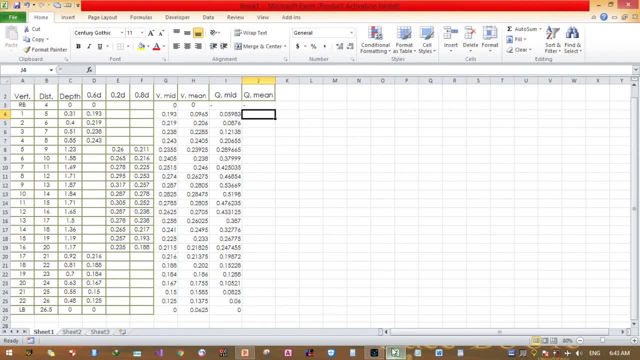 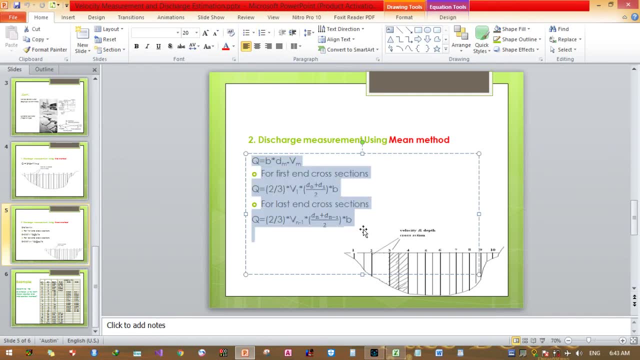 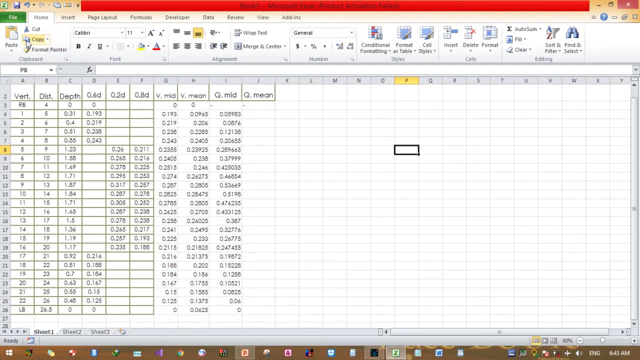 times width, so so we can convert this. so multiply with: here velocity one, velocity one: is this one velocity, not velocity one. they do not as well. so velocity not four mean is here velocity mean. and this one multiplies with this average: here damage average is here: gives one plus. 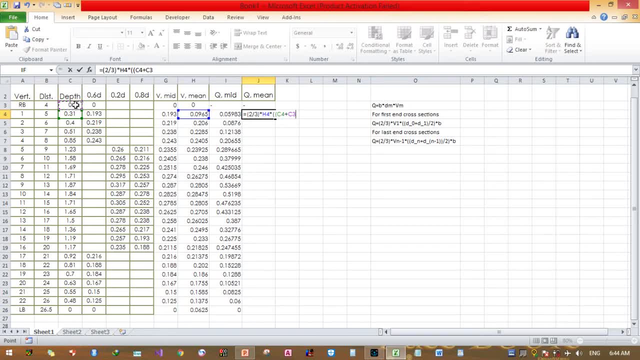 this notes times the width, which is one meter, which is five minus four. so you did that. now we have filled in such a way, now for the rest one. for the rest one, you can fill B times W times velocity. so here first equal sign, here, which is a constant one six minus five, one. seven minus six, one eight. 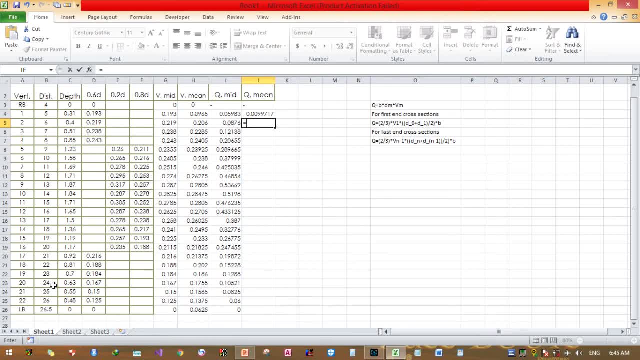 minus seven, one, nine minus eight, one in the constant till twenty five, twenty six here, sorry, and the last one with the 0.5 here, as you can see. so here: width, one meter times depth average. depth average here: this one plus this one, close to divide by two. close this depth times bracket velocity average. 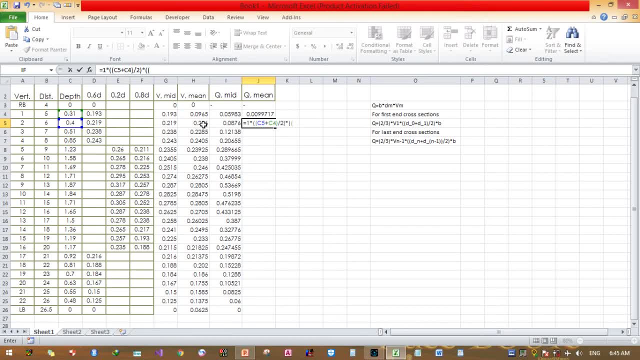 mean velocity average here. take this: P mean this one plus this one. close bracket: two divided by two. now we have finished the equation and hit enter, hit, enter. now, as you can see, we can drag till the end cross-section. but we can fill this in the cross-section with the equation with this one. 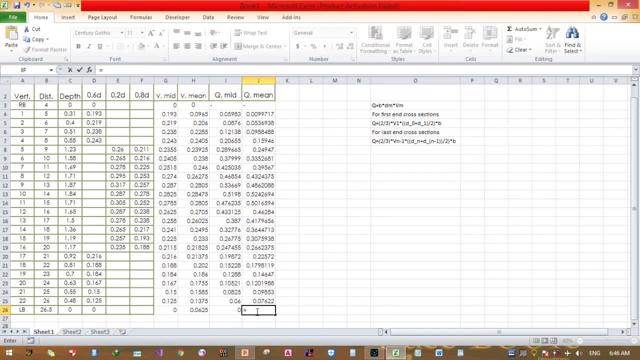 and which is equals to: but here the velocity, different two divided by three multiplies with velocity n minus one, not n. so velocity n minus one, velocity at n minus five is here, velocity at n is 22 and velocity n minus one will be, and velocity one is at 22. therefore, uh, we'll take this mean velocity and the velocity at n is this one, and 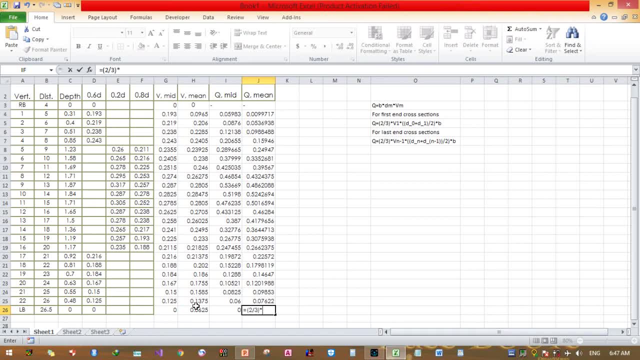 velocity at n minus one is this one. so so uh takes this velocity in the management times. this is average. this is average here. so this is the tips here, plus this one. close to divide by two close the average times times. here. the only thing remaining is uh tips or widths. so the width is: 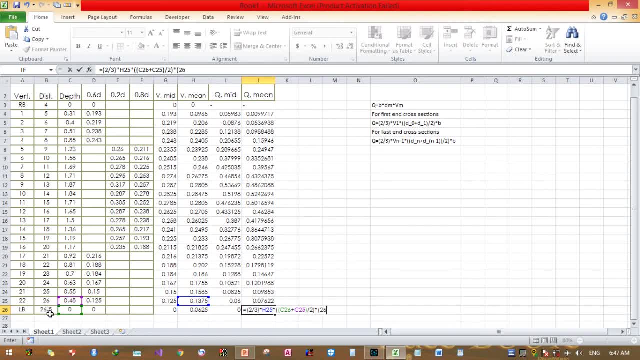 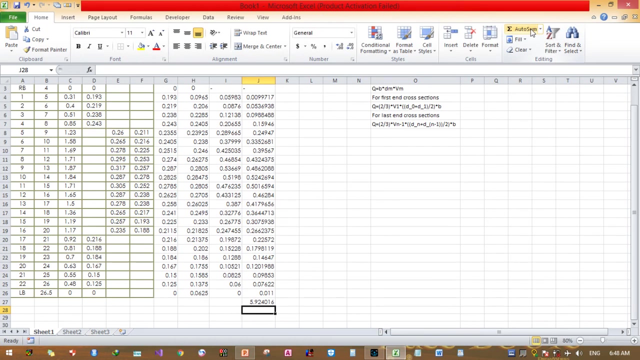 26.5, that is 26.5 minus 26 in the width, so you can multiply such a way and hit enter. finally, this is how we can uh calculate using midsection method and uh mean a meter, so we can compare by autosun here the value here: